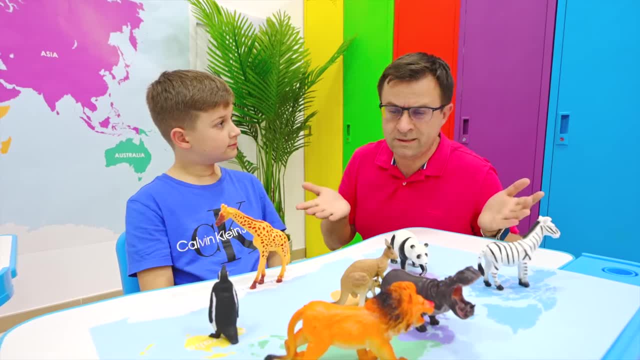 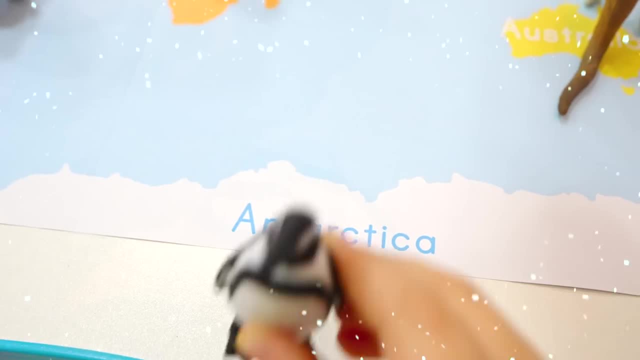 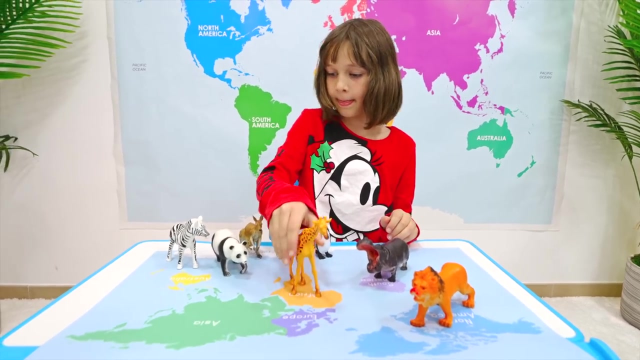 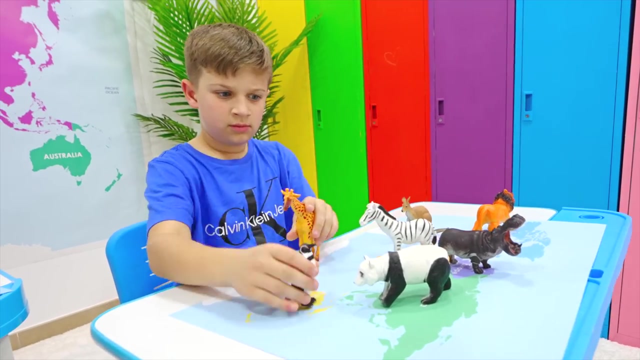 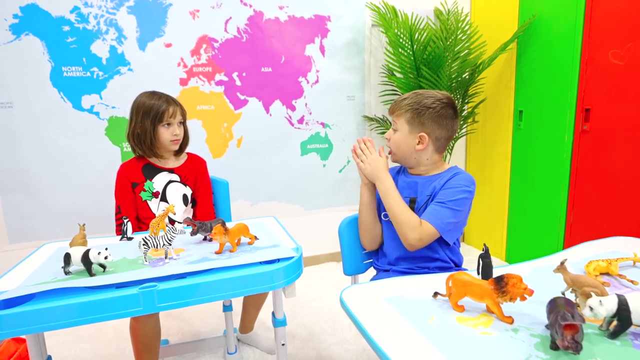 No, no, no, It's not correct. You need to think more. Ok, Ready, Uh-huh, Hmm, Good Super, I don't know how to do this correctly. I will help you. Yes, please, Ok. 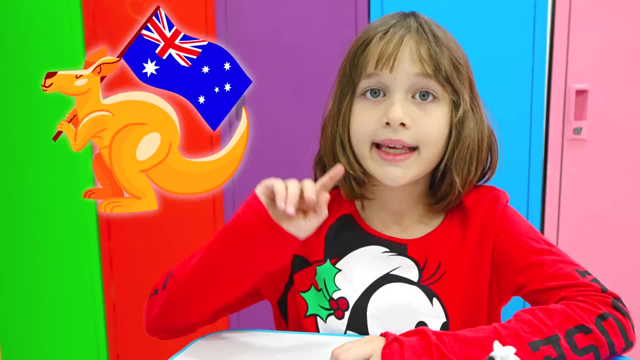 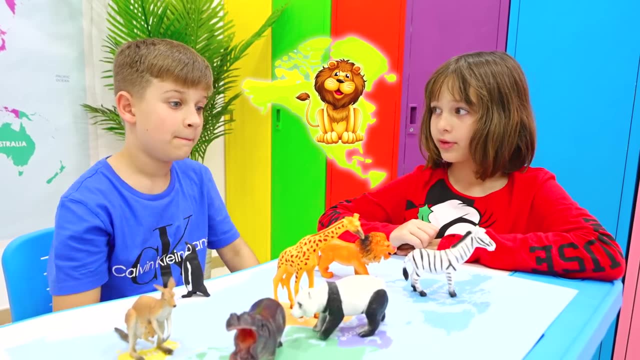 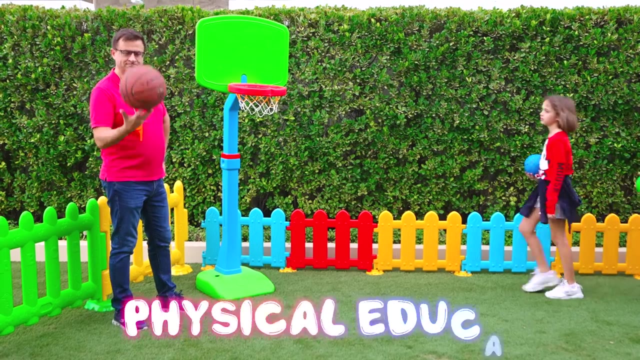 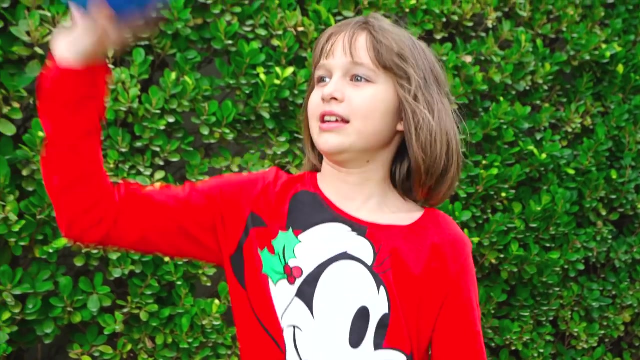 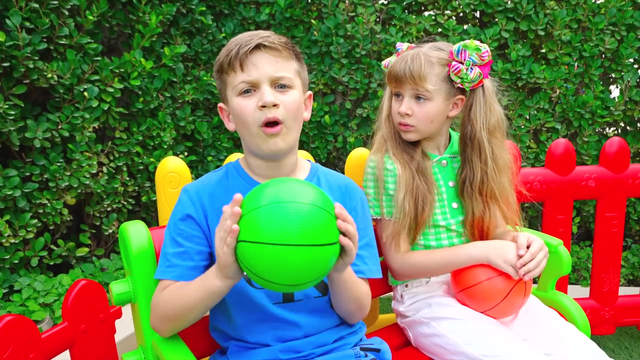 Giraffe lives in Africa, Kangaroo lives in Australia, Lion lives in North America. Yay, Today we will play basketball. Look, I will do it now One more time. Come on, You are doing wrong. First you must warm up. 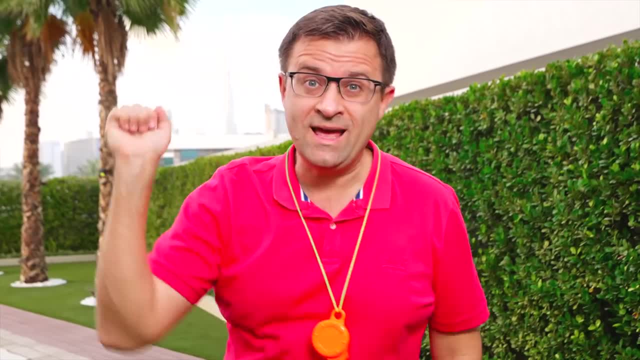 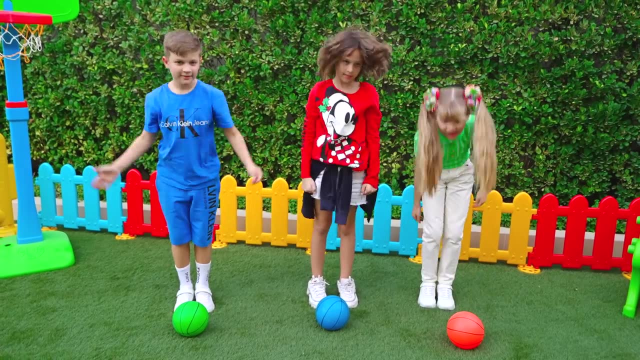 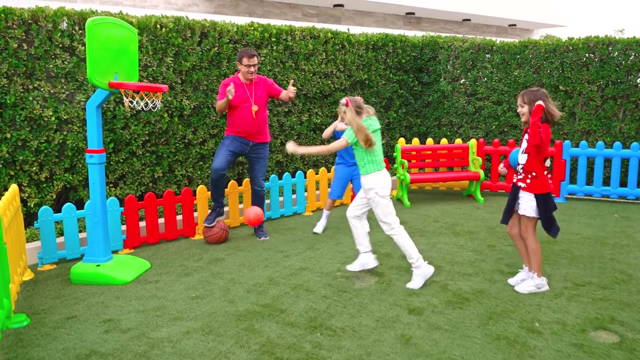 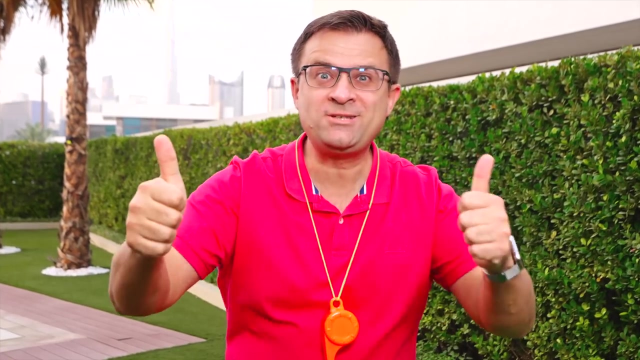 Exactly Roma. Let's start exercises. Ok, Yay, Yes, Yay, Yay, Now me, Yay, Wow, Yay, Great job, Come in. come in Sit down please. Music lesson: Uh-huh. 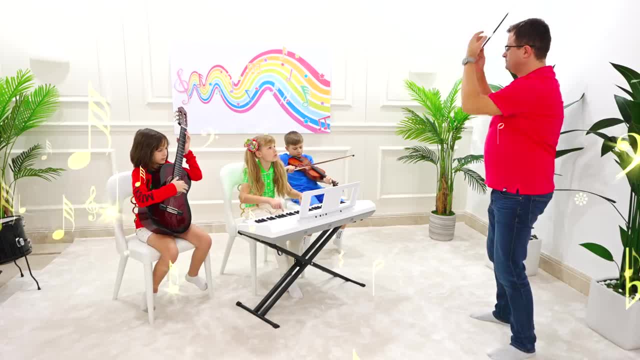 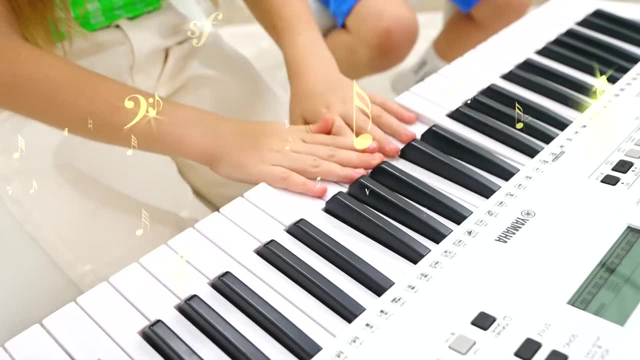 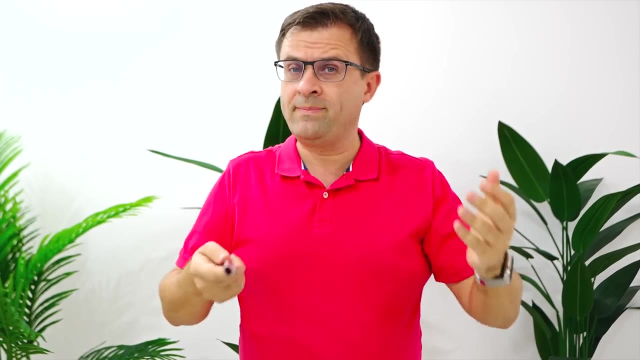 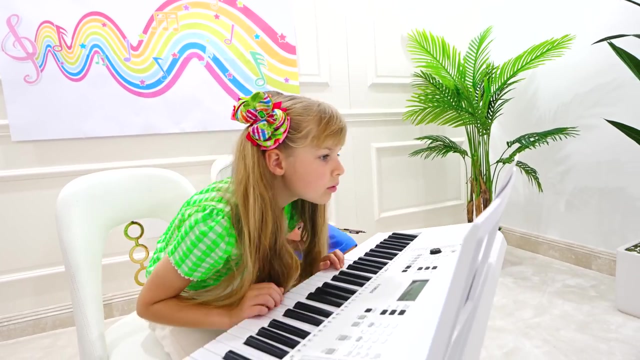 Let's start. Hmm, Hmm, Hmm, Hmm, Stop, stop, Diana. what happened? I can't do this. Don't worry, This will help you. Uh-huh, That's not all. Great idea, Super Ok. 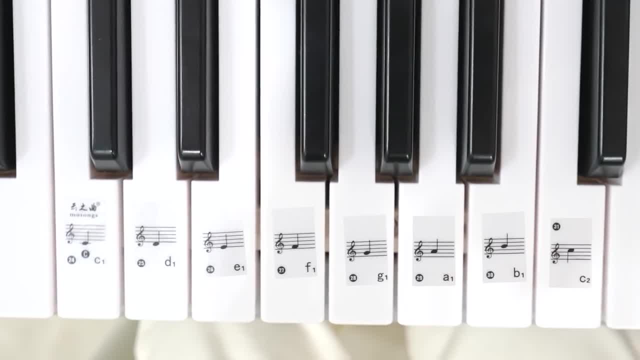 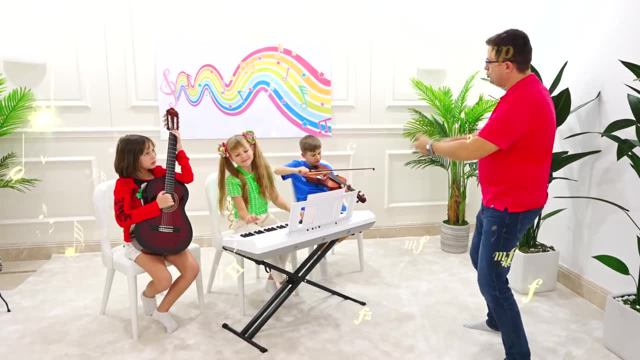 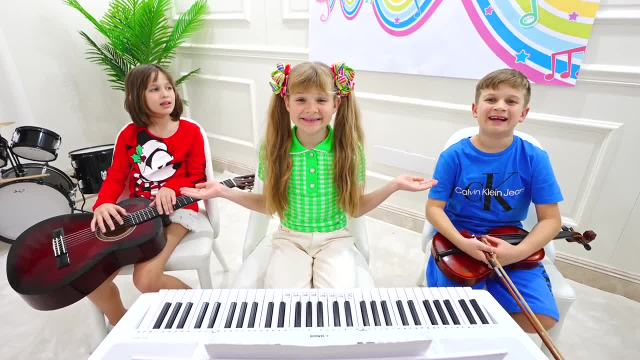 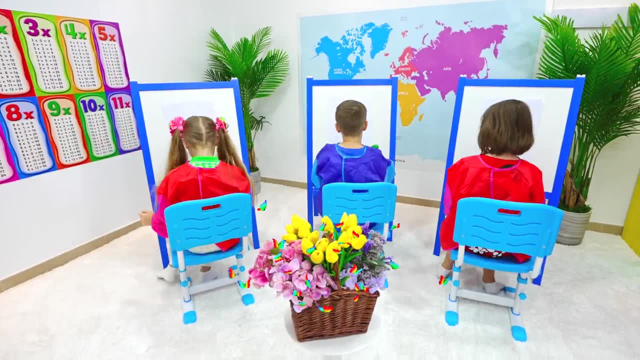 Yay, Excellent, Thank you guys. You're welcome. You're welcome, You're welcome. Art lesson: I like arts, Me too. Let's go. Awh, Hmm, Lalalalalala, Lalalalalala.